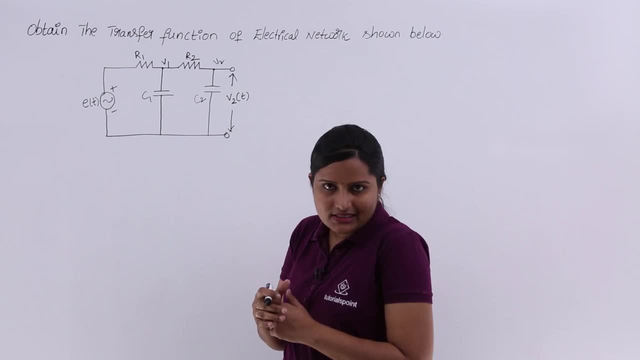 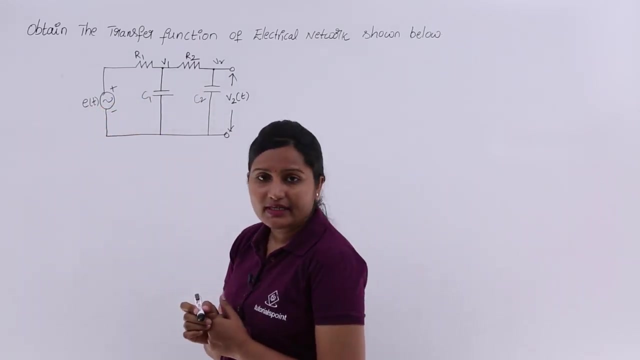 addition of all the voltage, all the currents entering that node, is equivalent to leaving. So addition of all all currents I am going to consider So here, coming to this, R 1, V 1 minus E of t, divided by R 1, will be the current flowing through that R 1.. 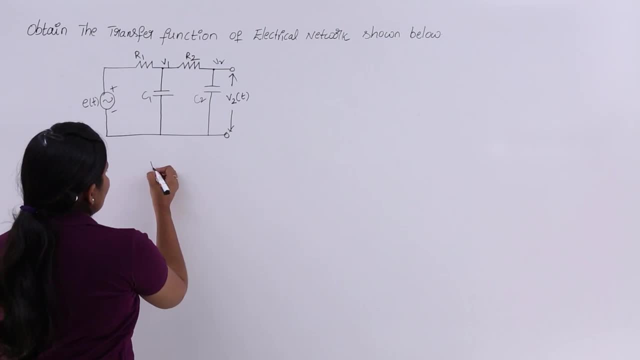 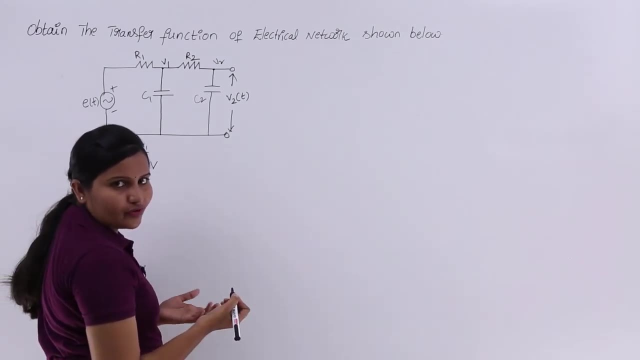 So current flowing through that R 1 is equivalent to: So I am writing at node node 1, node V 1, V 1 node you just treat like V 1 node with voltage V 1.. So I am writing the current. 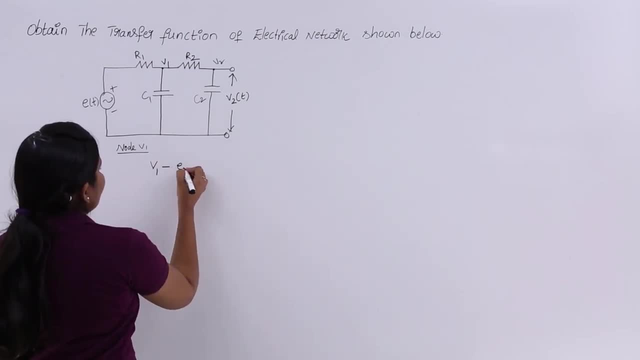 through this: R 1, V 1 minus E of t, V 1 of t. I am writing. So V 1 of t minus E of t, divided by R 1, will be the current plus. So one capacity is attached to the same node. So 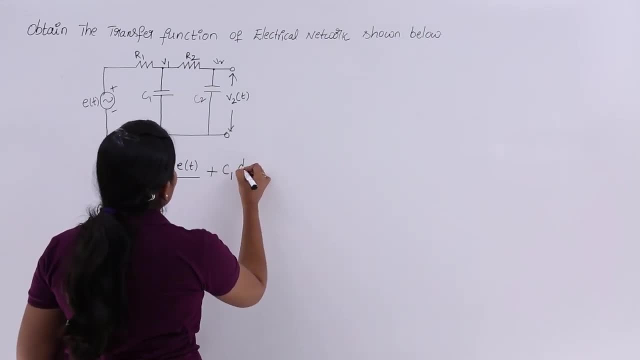 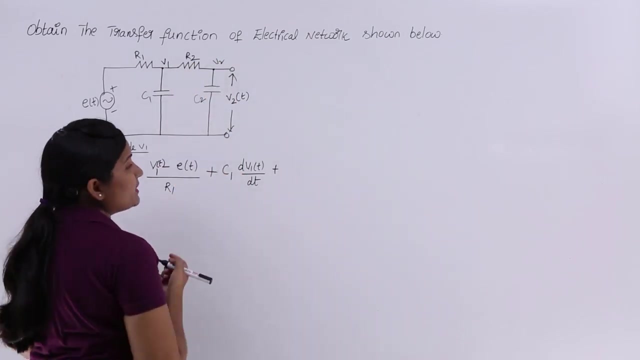 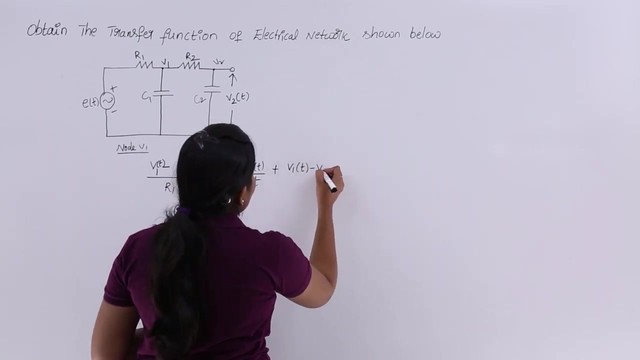 current through that capacitor is equivalent to C 1 into d V 1 of t by dt. this is the current through capacitor. Similarly, another resistor is there attached to that node. So V 1 minus V 2 by R 2 will be the current passing through R 2.. So here V 1 of t minus V 2 of t divided by R 2 will be: 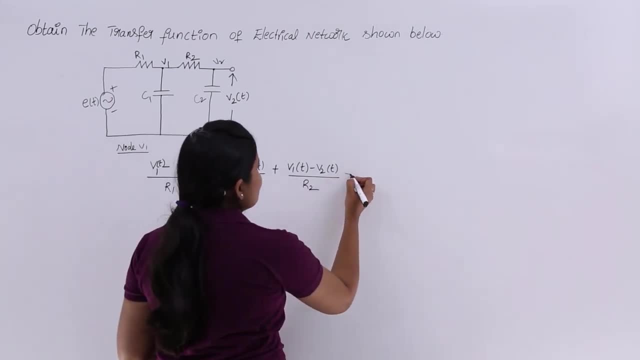 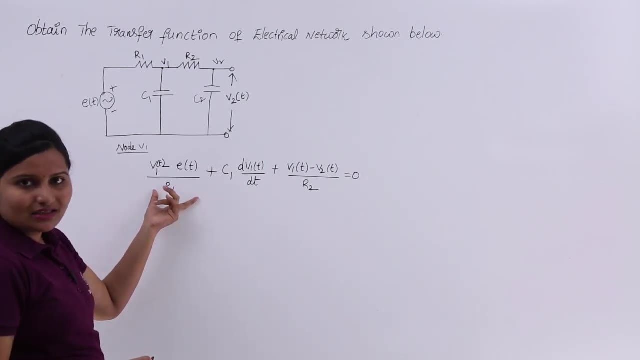 the current in this R 2.. So this is equivalent to 0,. this is equivalent to 0.. So now here I want to consider Laplace transform on both sides. What we need to ensure, We need to get the transfer function of the system, Transfer function of the system- is nothing. 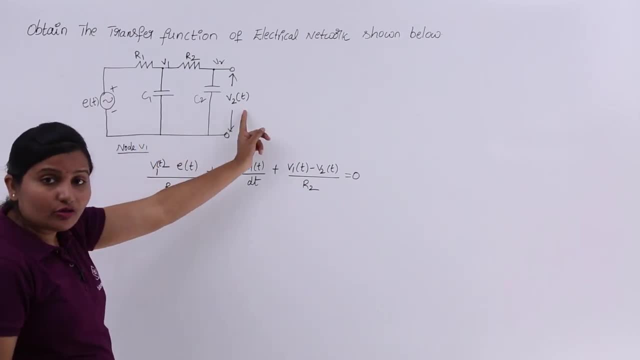 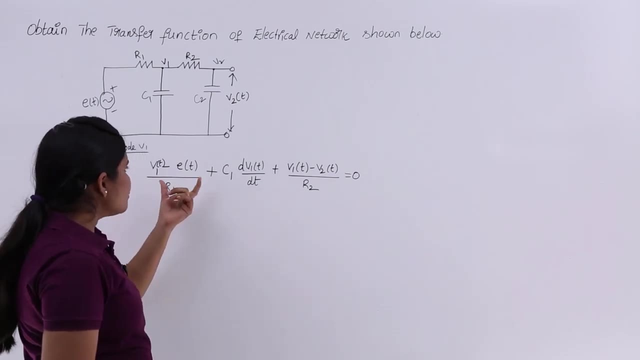 but output transform by input transform. Here the output transform will be V 2 of S and input transform will be E of S. So here to get that S domain, after writing current equations, we are going to write Laplace transform for that equation. Take Laplace transform on both sides for this equation, then you are going. 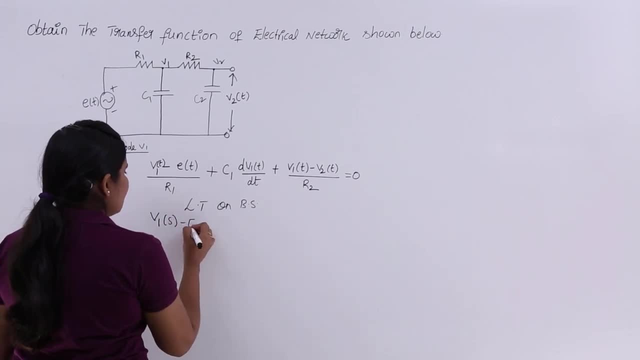 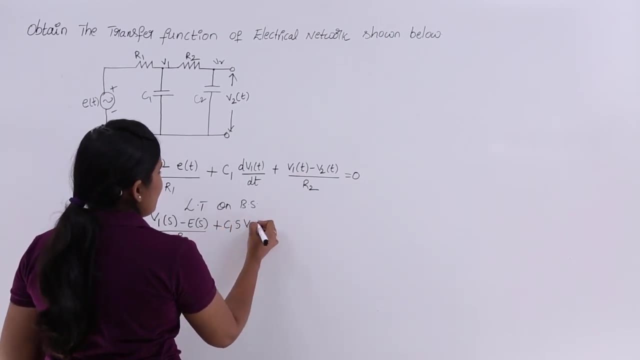 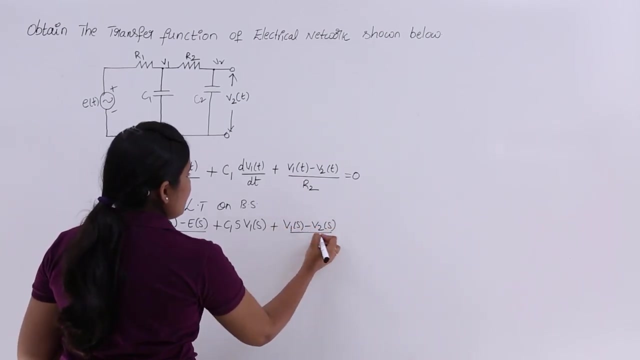 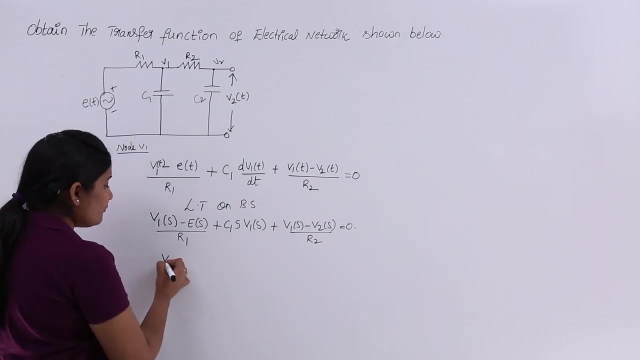 to get V 1 of s minus E of s, divided by R 1 plus C 1 s, into V 1 of s plus V 1 of s minus V 2 of s divided by R 2 is equivalent to 0.. Now I am going to take common of V 1 of s. 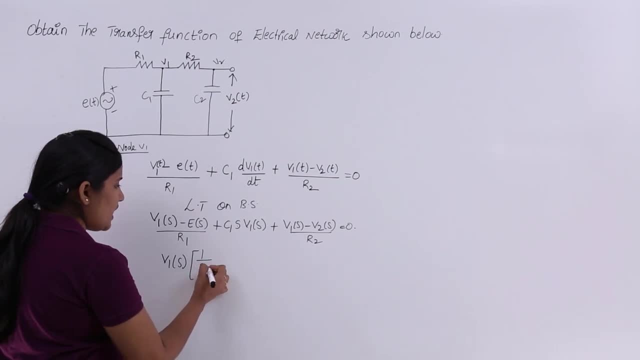 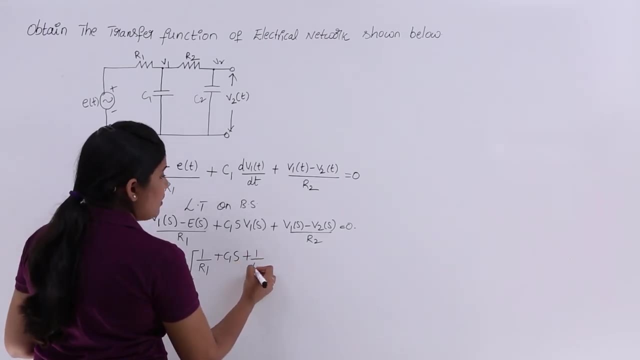 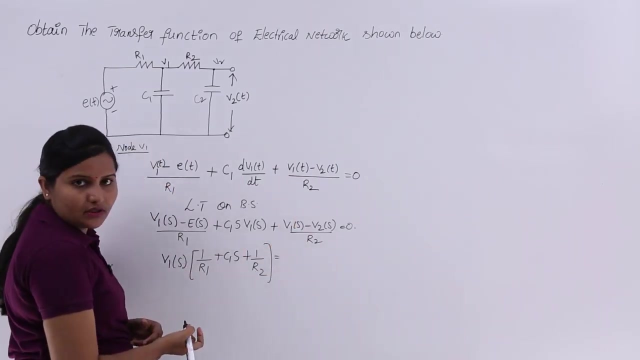 here V 1 of s into 1 by R 1 plus. So here I am having C 1 of s plus 1 by R 2. So here I am having 1 by R 2. Remaining terms are having minus. So I want to send them that. 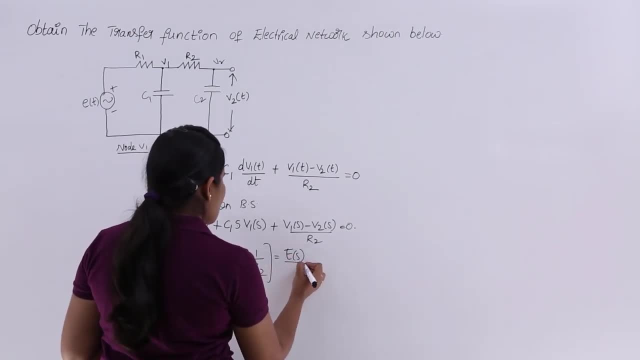 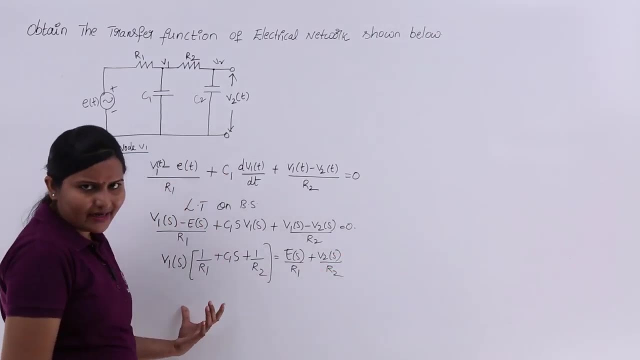 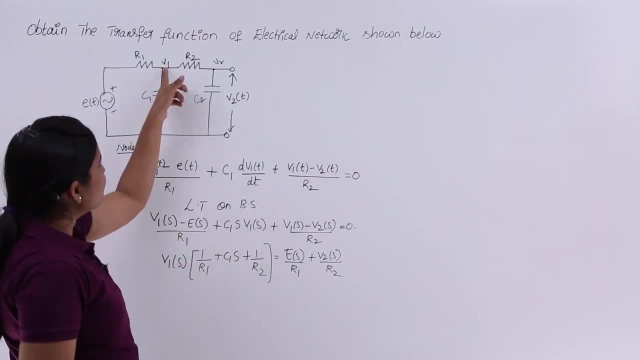 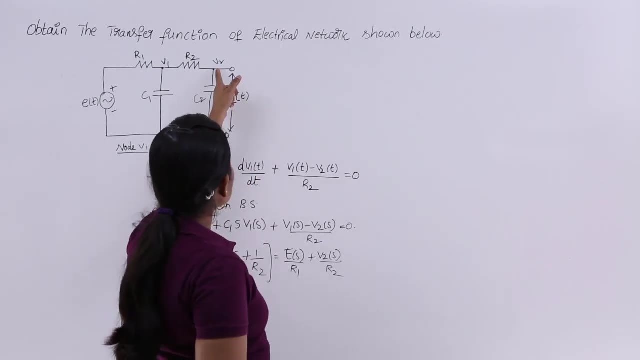 So this is the equation related to node this node, first node. At node 2, similar equations I am going to write at this node. So this node is having connection with this R 2.. So I am again applying KCL at that node. So here the current flowing through R2.. 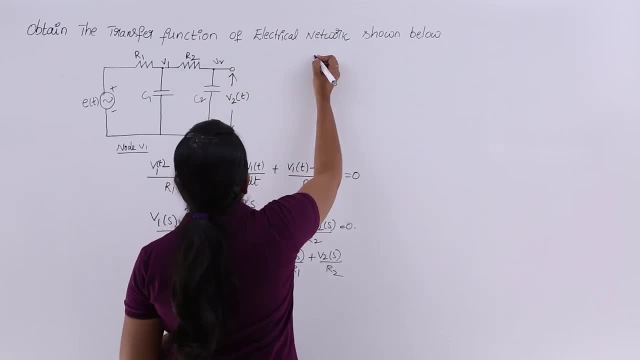 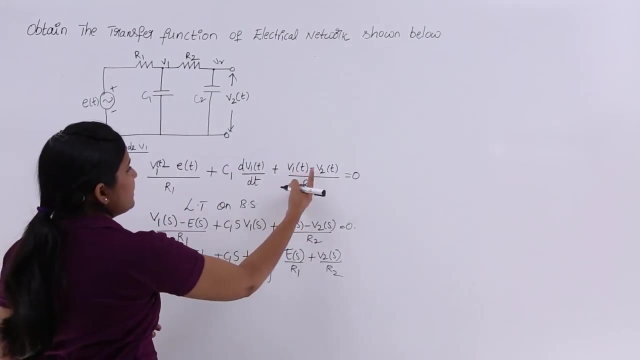 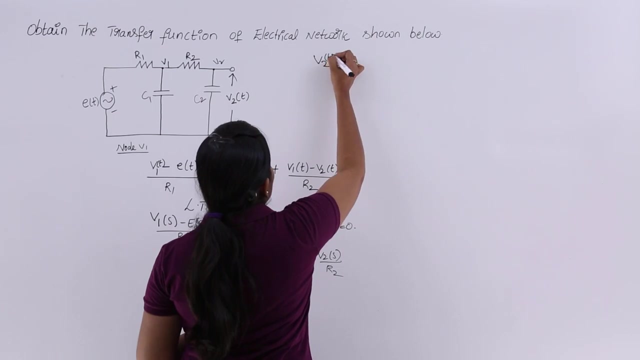 So R 2 is from this side, is V 2 minus V 1.. So here U return. So here: V 1 minus U, V 2 U return. So similarly you need to write V 2 minus V 1, that means V 2 of t minus V. 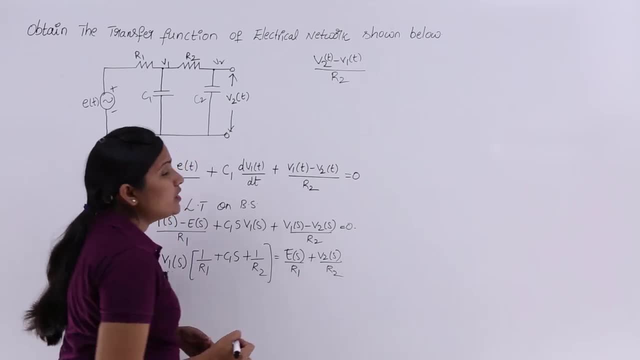 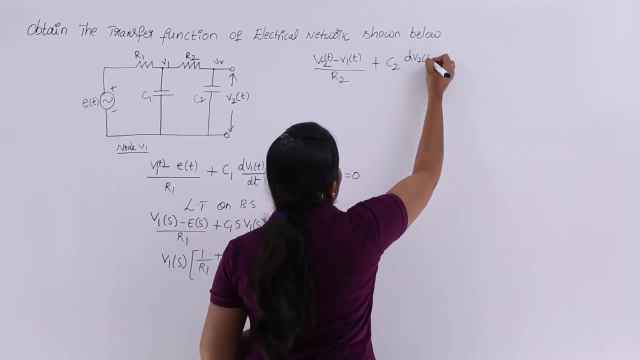 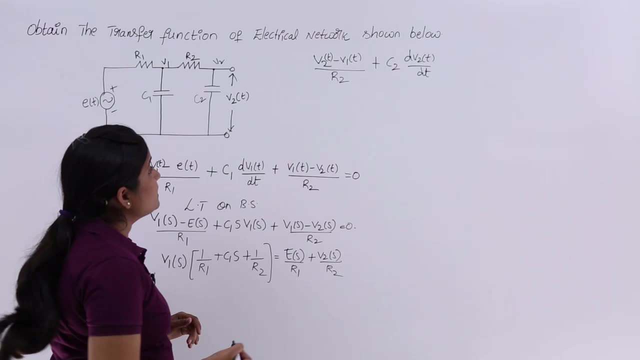 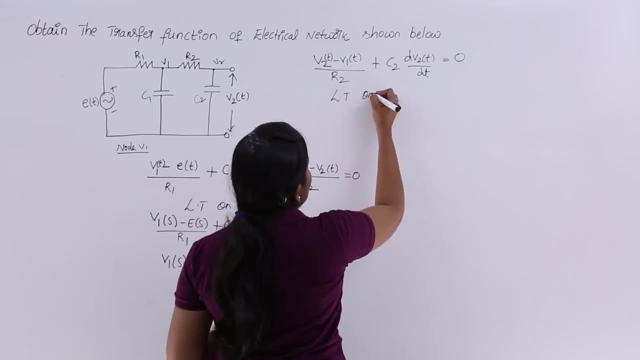 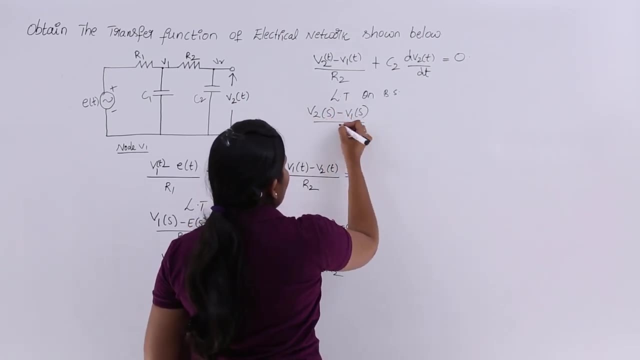 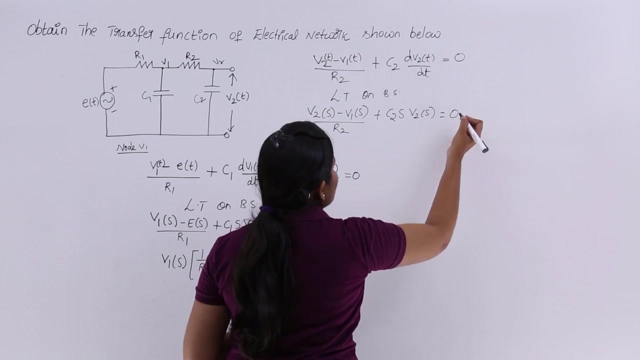 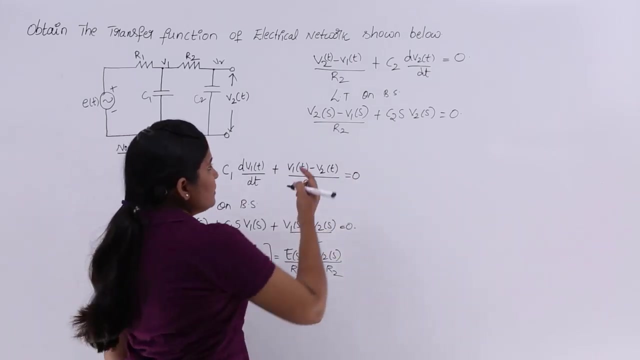 Now again, apply Laplace transform on both sides. So you are going to get v2 of s minus v1 of s, divided by R2 plus c2 s, into v2 of s. When you are having differentiation, if you consider Laplace transform, then you are going to get s into v of s. So now I am going 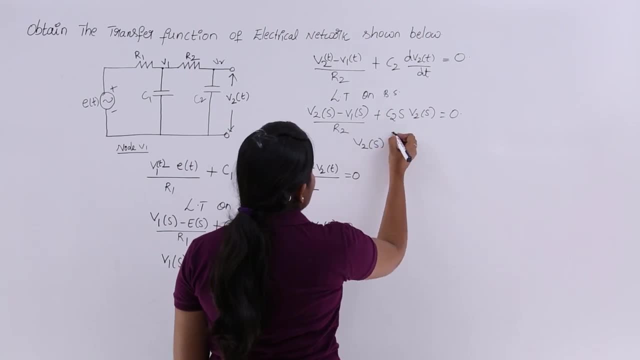 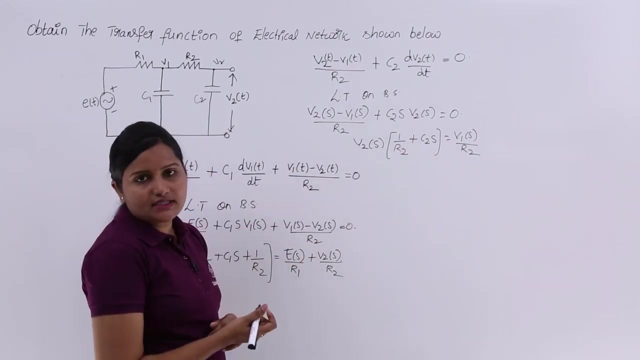 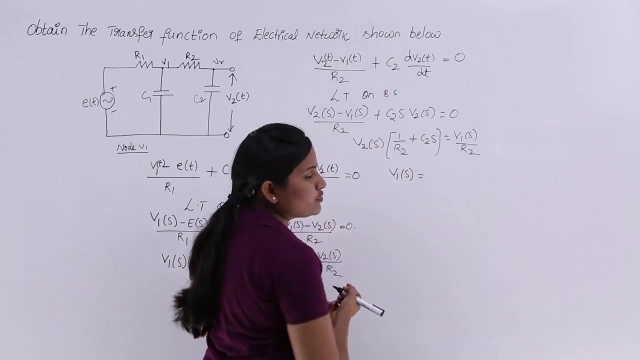 to take common of v2 of s. v2 of s into 1 by R2 plus c2 s is equal into v1 of s divided by R2.. If you want v1 of s, then so v1 of s is equivalent to: I am sending this R2 this side, So here. 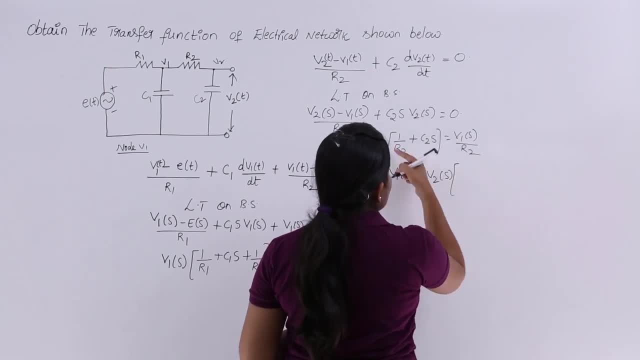 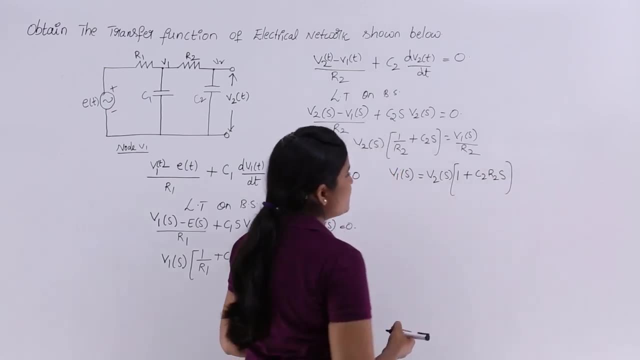 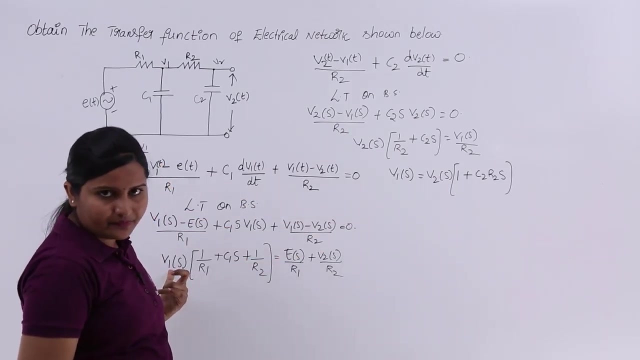 v2 of s into. if I multiplied this R2 to inside 1 plus c2 R2 s, So that will be c2 R2 s. I got v1 of s value, then I can substitute. So here I am substituting that v1 of s here. So here I am substituting that v1 of s in. 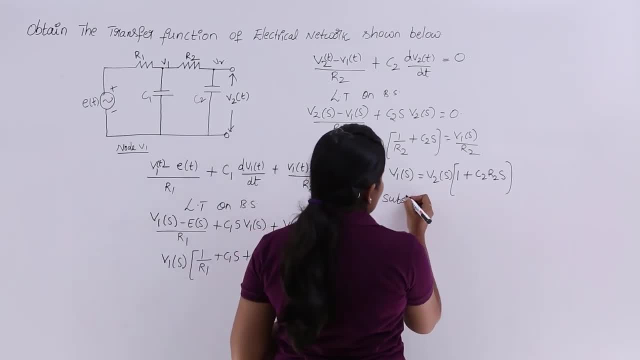 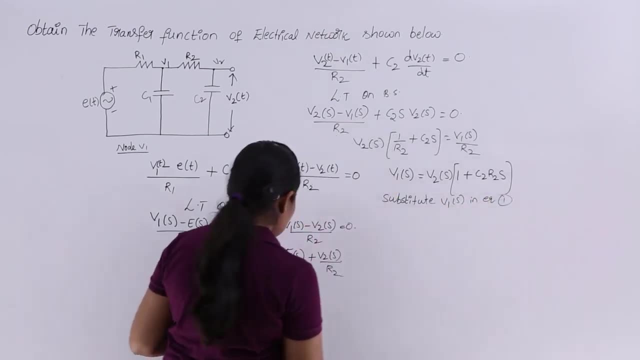 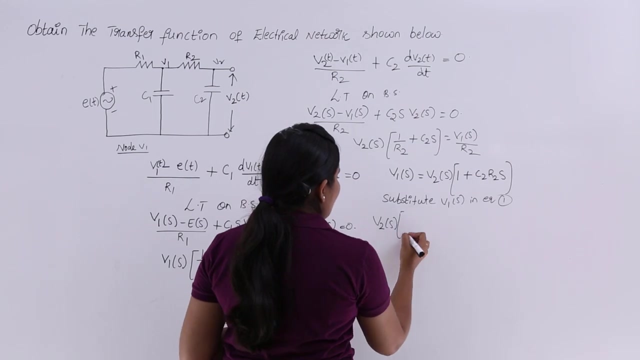 this equation substitute: substitute v1 of s in equation 1.. You can consider this as equation 1. then you are going to get So v2 of s into 1 plus c2 R2 s in place of v1 of s. 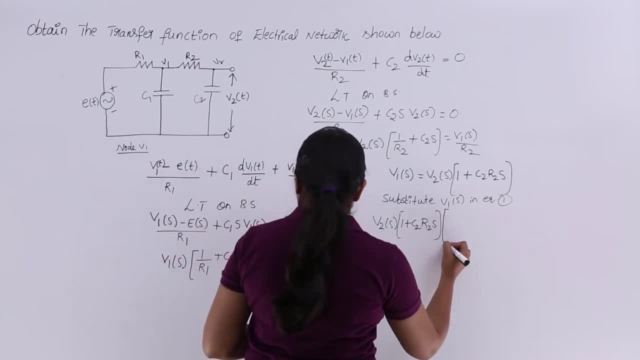 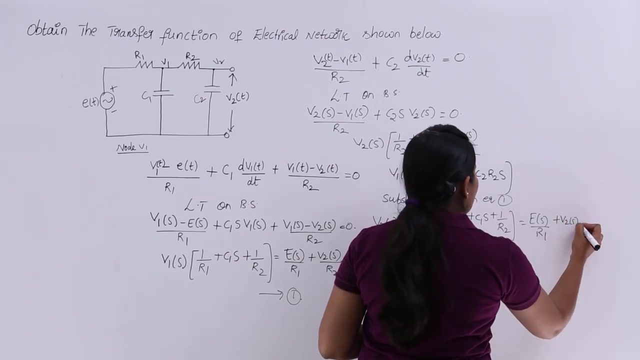 So I consider this remaining. I need to write: So that is, 1 by R1 plus c1 s plus 1 by R2 is equivalent to: So E of s by R1 plus v2 of s by R2.. So what I require, I require. 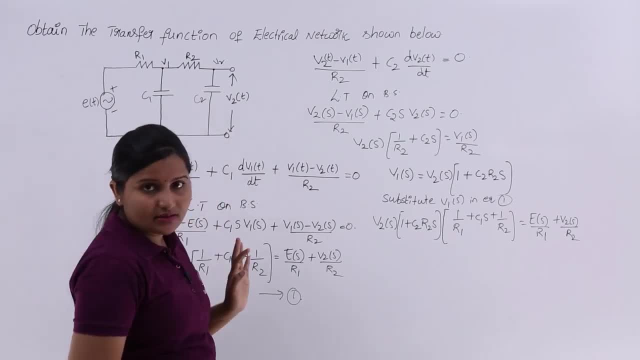 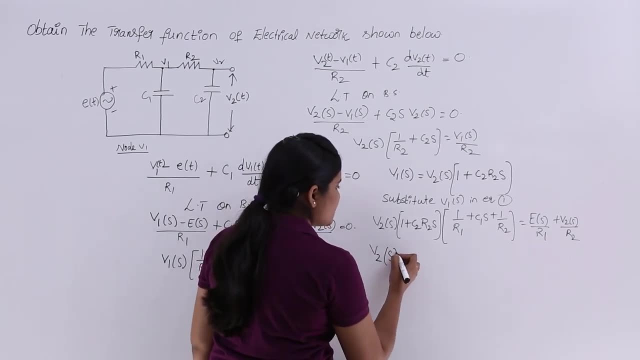 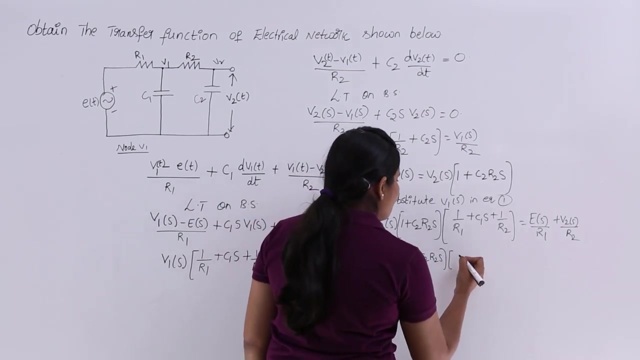 finally, v2 of s by E of s to get the transfer function. So I am sending this, So I am sending this v2 of s this side and taking common of total v2 of s. v2 of s is equivalent to 1 plus c2 R2 s into 1 by R1 plus c1 s plus 1 by R2 minus 1 by R2. 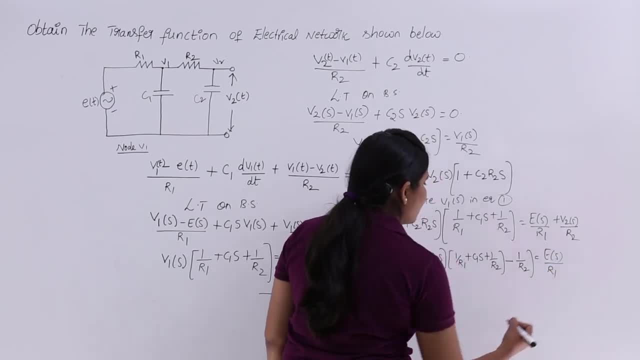 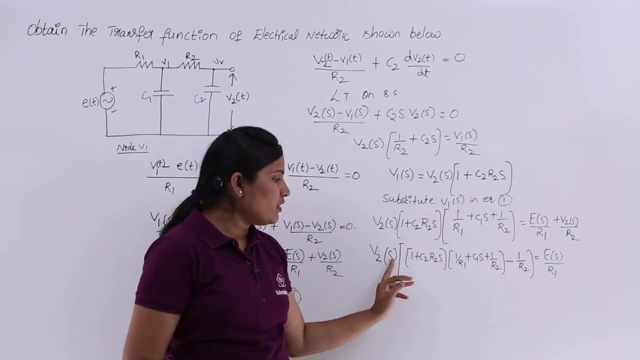 is equivalent to E of s by R1.. You can see v2 of s is equivalent to. I send this also to this side and take in common of v2 of s. If I take in common of v2 of s, I am going to. 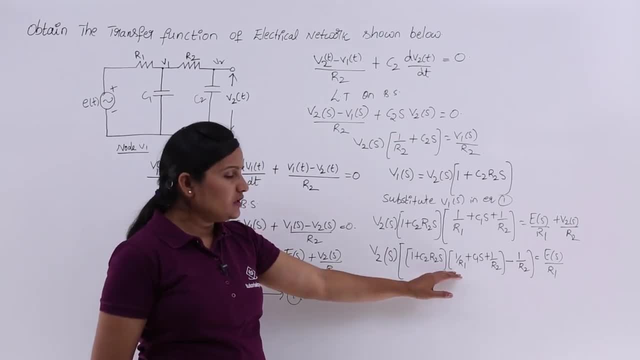 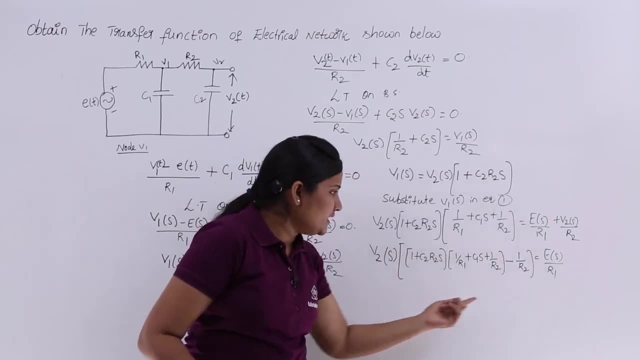 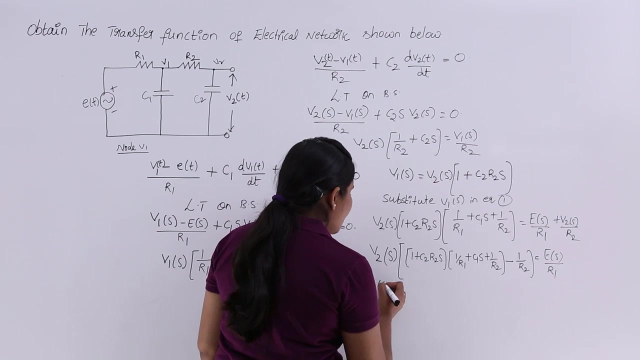 get like this: Now my equation can turn into transfer function by taking So v2 of s by E of s. So now I am taking like that v2 of s divided by E of s is equal into So: 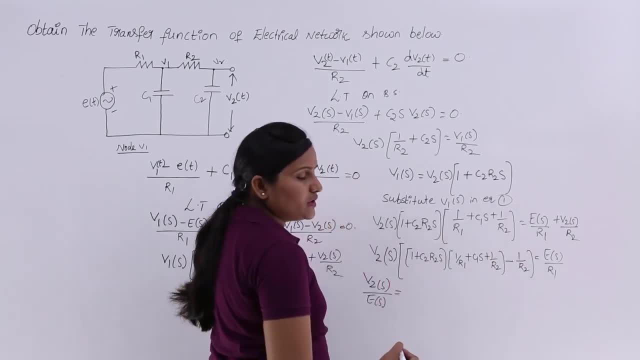 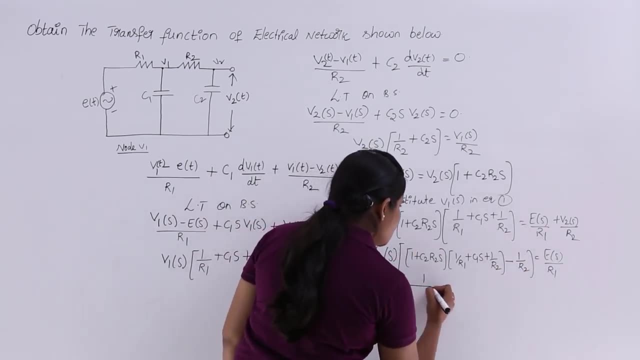 I am taking like this: I can send my equation to this side. So that means. so if I sent like this, I can send to denominator- That means 1 by R1- into. so you can write everything here: 1 plus c2 R2 s. So 1 by R1 plus c1 s plus 1 by R2 minus 1 by R2.. If you want to, 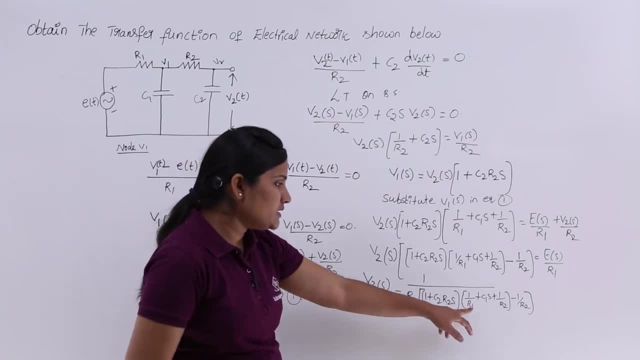 If you want to simplify this equation, you can simplify. that means, if you want to cross, multiply this R 1, R 2, and if you want to send this R 2 to denominator, you can send. So here the form of transfer function will be like this: 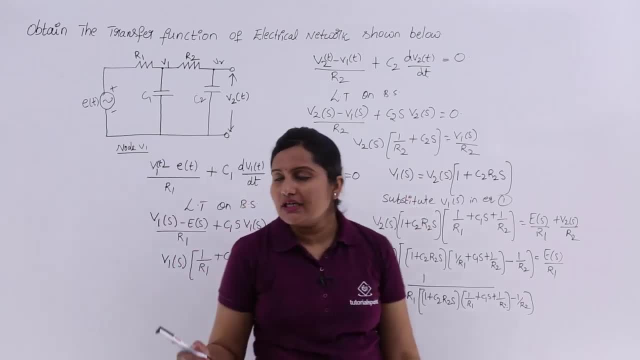 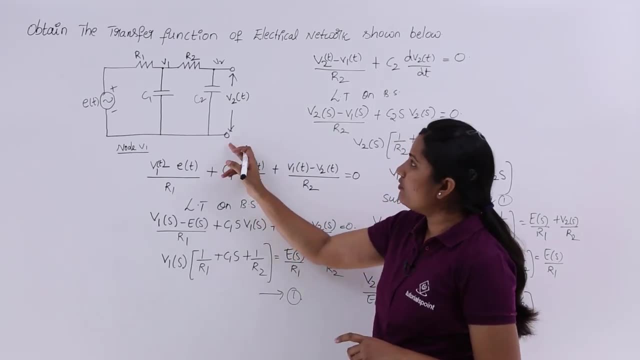 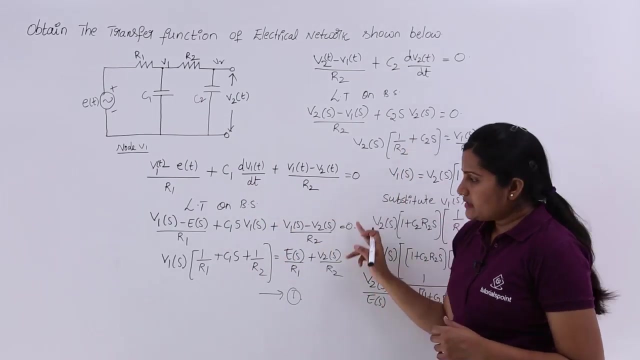 So this is the transfer function related to this electrical network. What we need to do means we need to consider the node equations. So at node 1 and node 2 I applied current equations. So here I considered that equations and I substituted one equation in another equation. 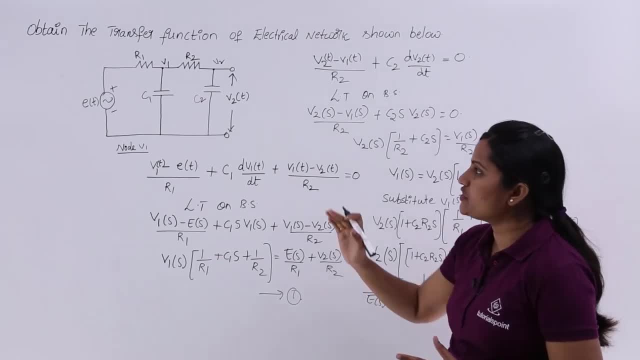 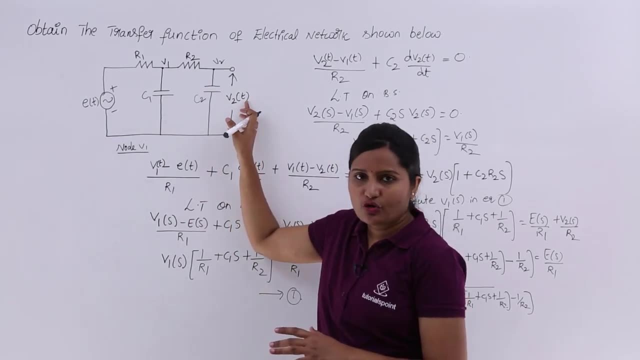 I am going to get this form. So to get the transfer function always we need to take output transform by input transform. Here in this circuit, output transform is V 2 of S and input transform will be E of S By taking V 2 of S by E of S. 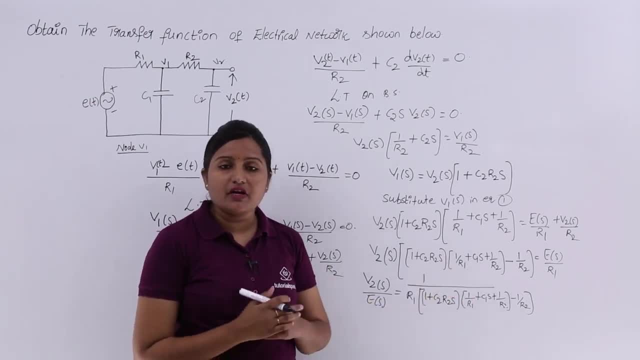 Then you are said to be at transfer function of this network.